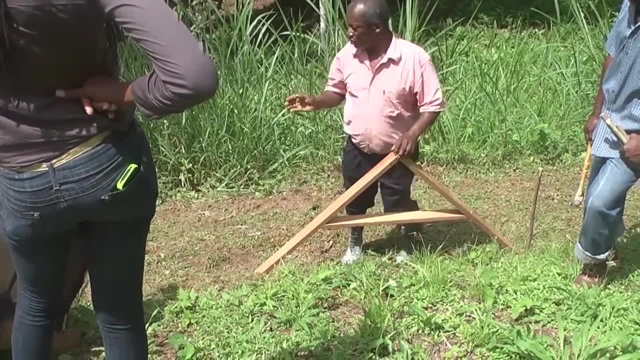 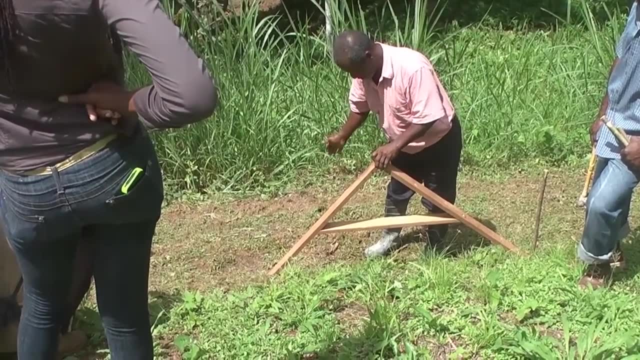 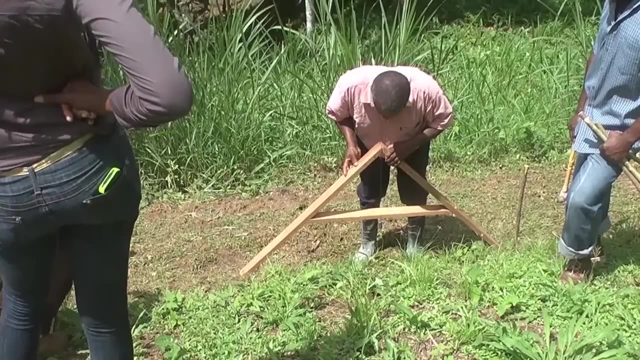 So everybody understand the word contour, Which means you're going same level around the hill, right? You're not going like this. This will be lower down, This will be too high. How you know the level When this plumb here falls direct on the mark. 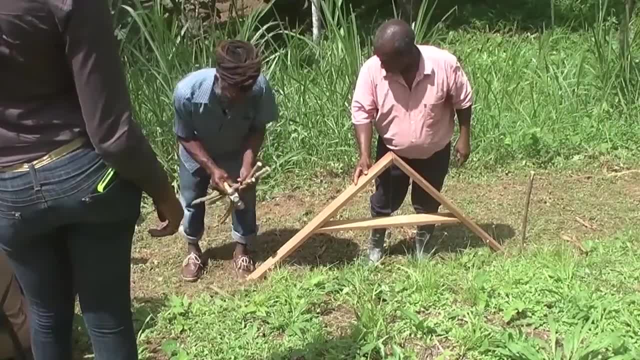 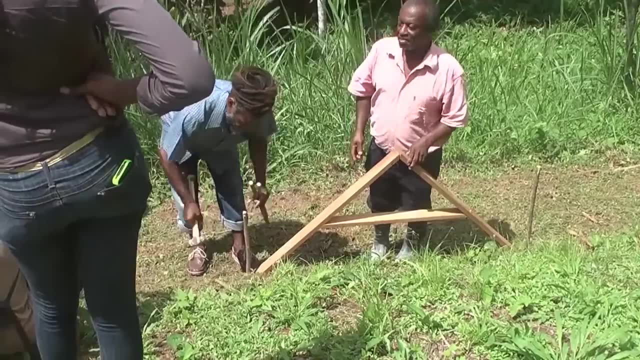 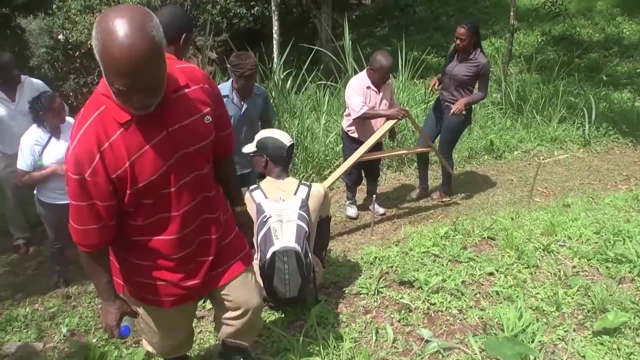 Right, Put a stick at the end. there You're sticking out your plot because you're going to put a mini terrace here or a contour drain or a high-brow terrace. Somebody will give me the next level here. I volunteer, Plumb up in the center. 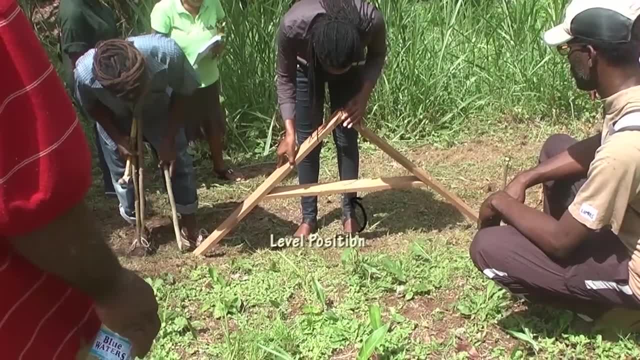 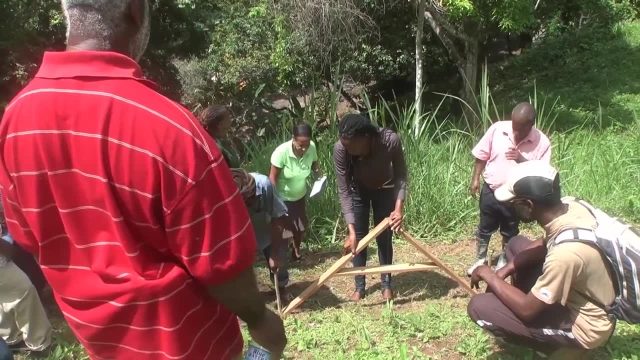 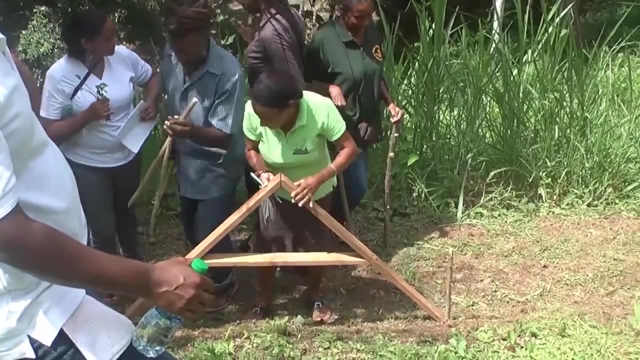 Yeah, How far you cut to me. Ah, finish again. Yeah right, All together on the mark. Stick Next person, Stick it from the next again. Yeah Right, Leave it. Plumb Three, Four again. 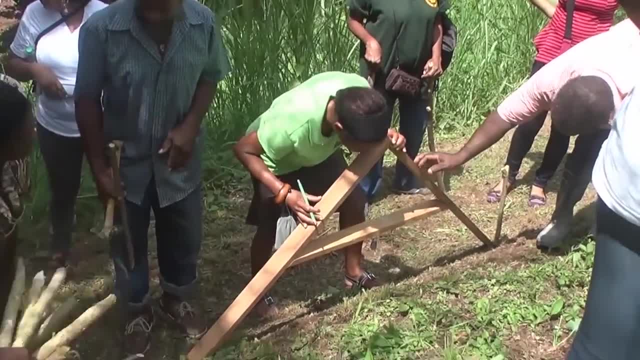 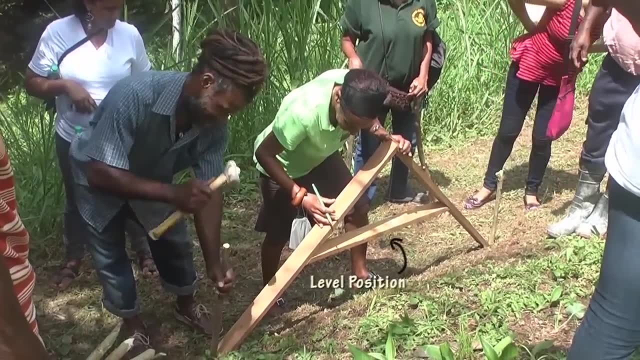 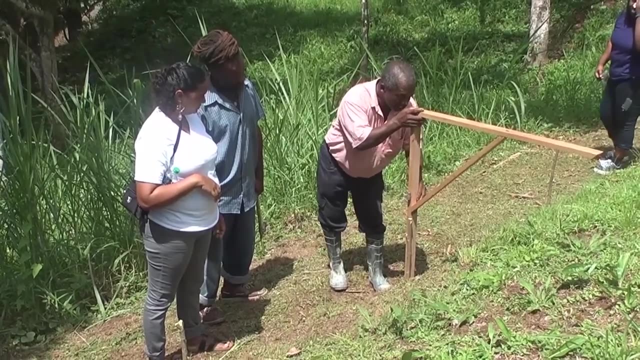 I love you Right, See the armor. Right, that's a go. So these are re-owning. I say Next, we need four more sticks. Right, you can work with that. Now I'm going to spy here Straight at the soil level here. Okay. 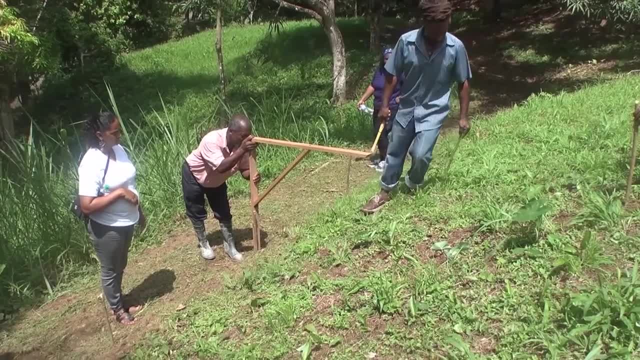 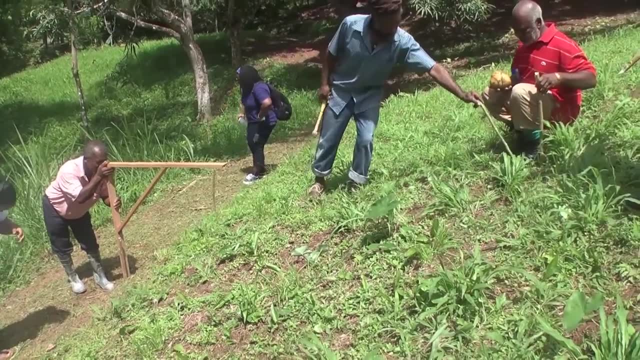 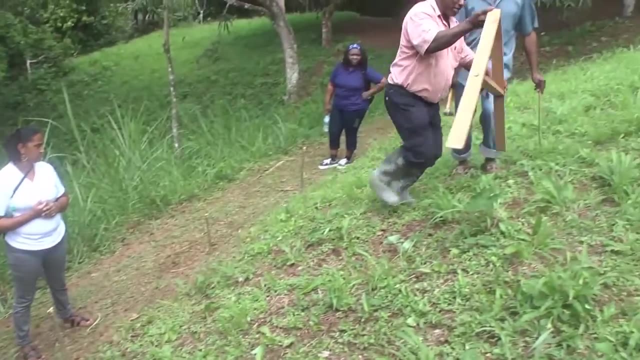 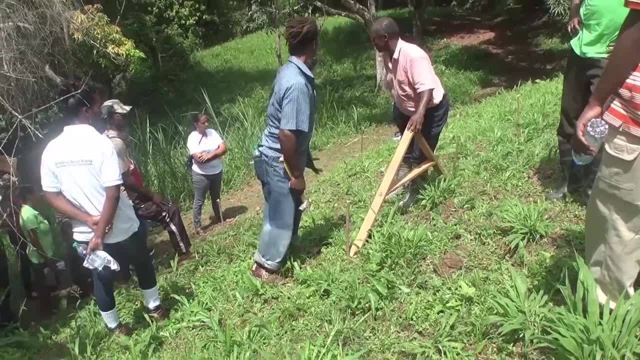 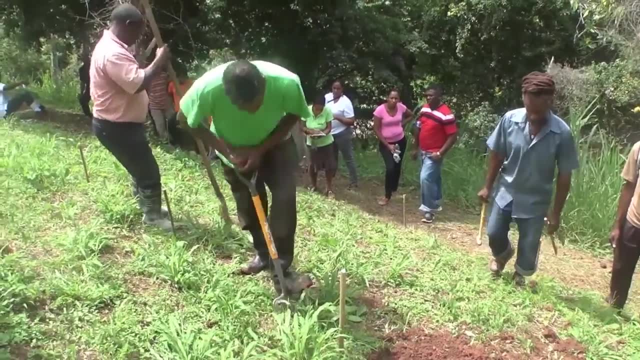 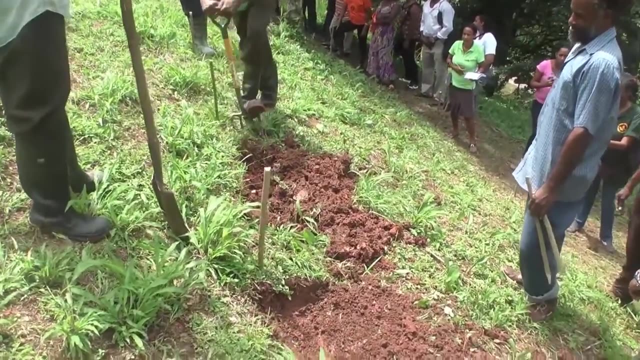 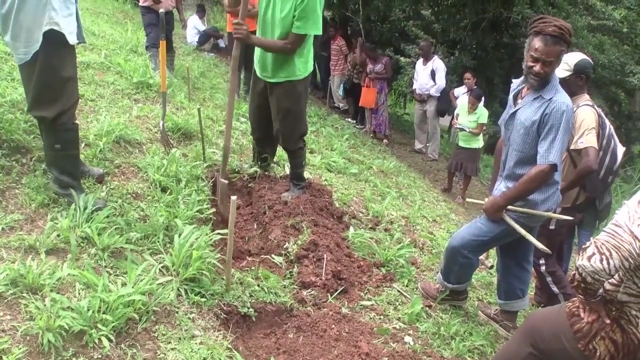 These mini terraces will be further up, So Let's construct a contour drain now. We'll do it right here. Right, this is a drain. This will be like 25 feet, 25 feet apart, So the drain is deeper Than the terraces. So what will happen with this? 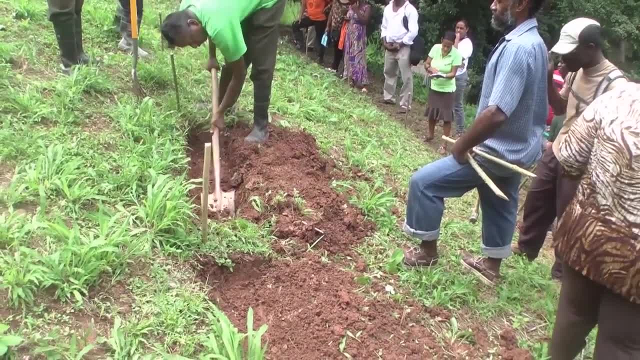 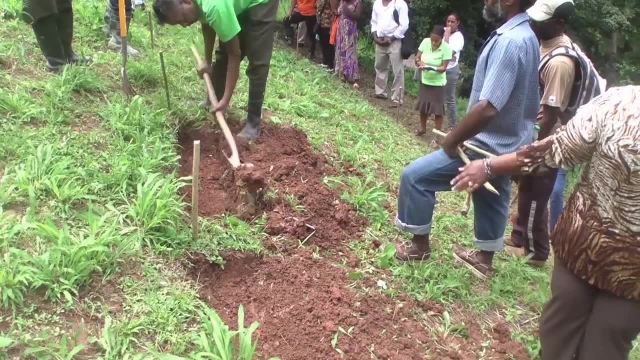 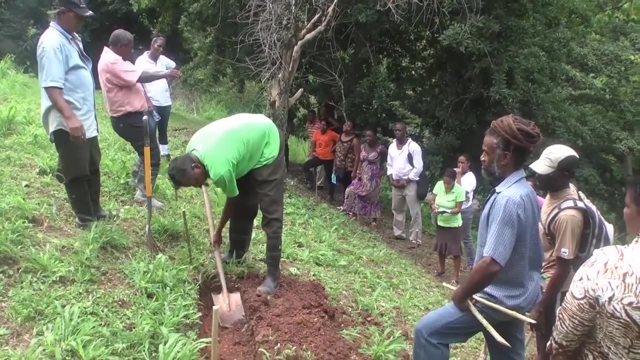 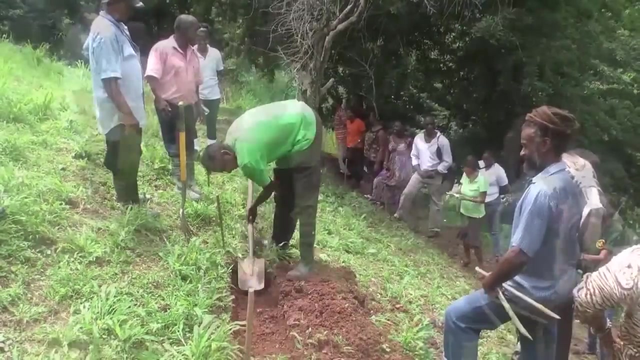 These contour drains Will drain On either side And go into the, The mini, The gullies And the mini streams With the check dam. So you have slowing down this way, You have slowing down that way And when they go into the check dam, More slowing down. It says. 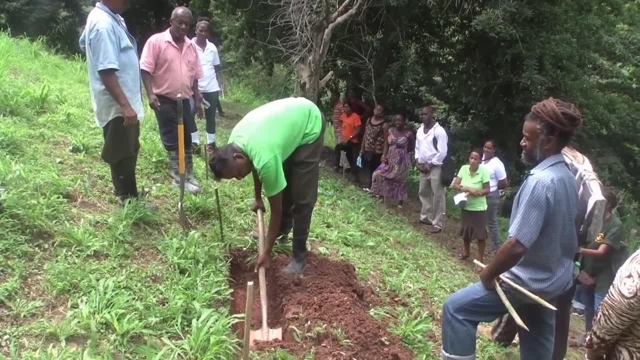 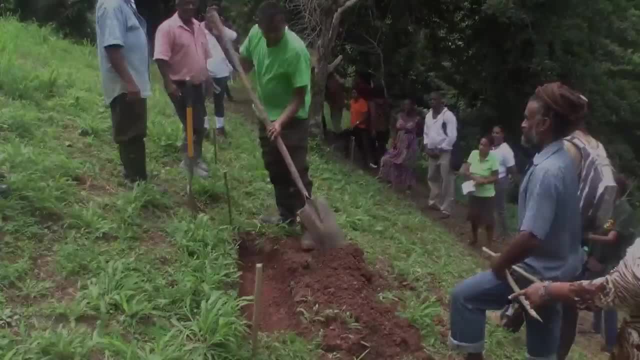 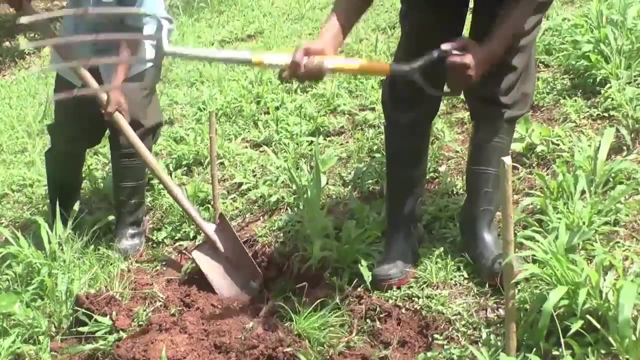 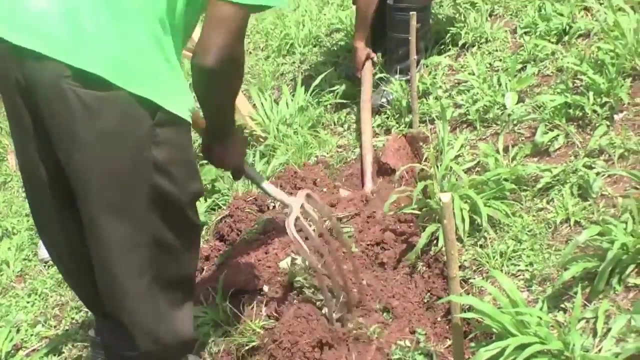 Right, Right, This is what it is, And space is scarce, So you're going to plant some okra or something On the edge here. Go back here And to this tree. Take a little more by this tree. Take a little more by this tree. Go ahead, Take a little more. 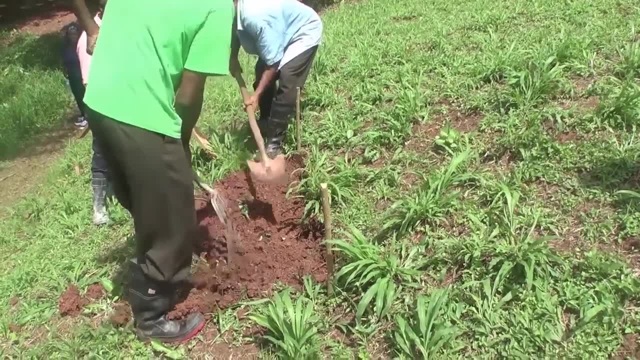 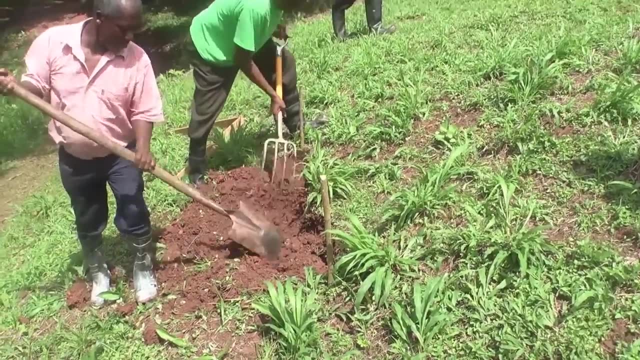 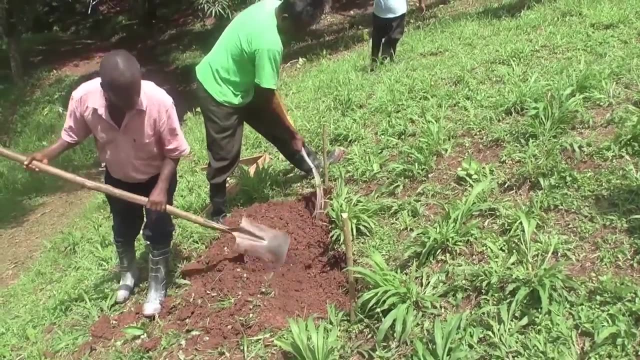 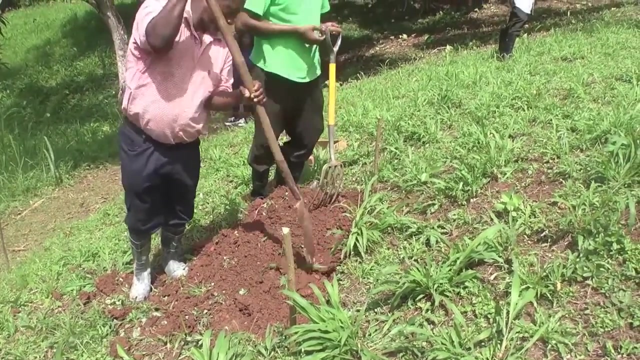 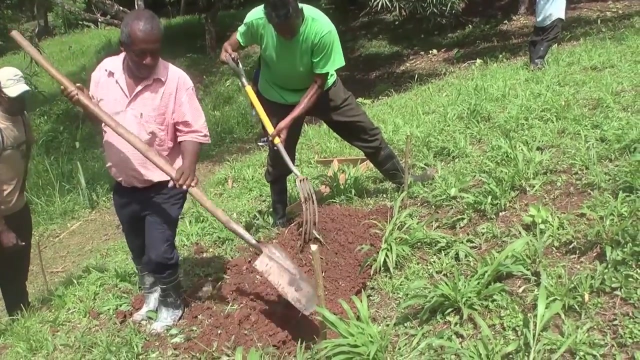 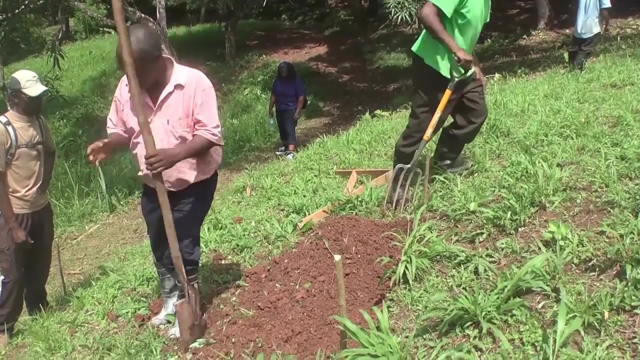 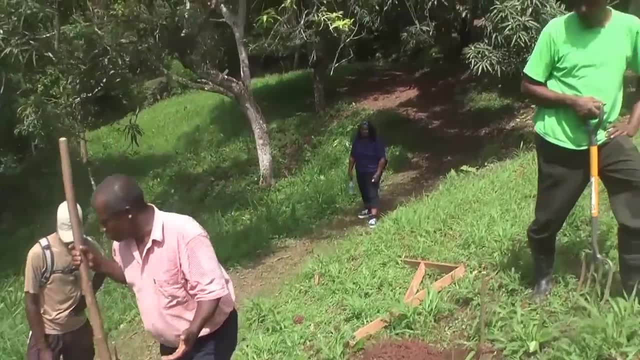 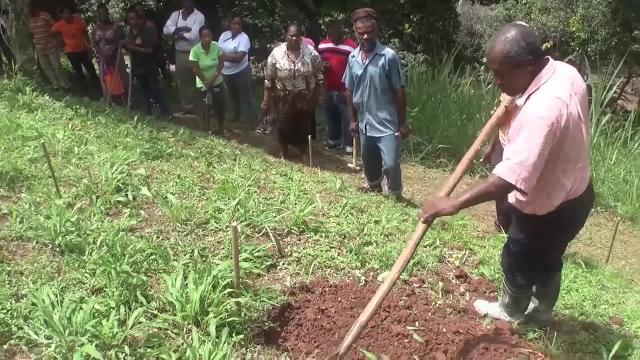 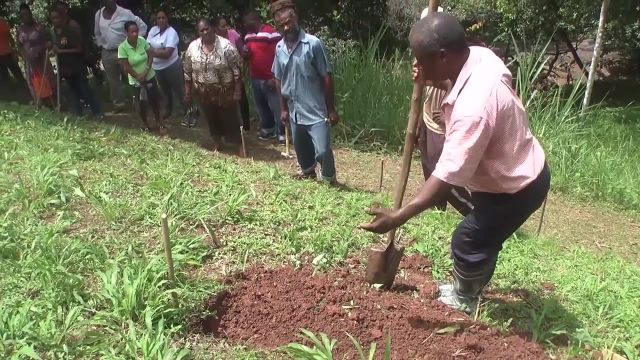 Because we really don't want to disturb too much soil. At the same time, you want to get to use the area right Water coming down this way- Remember- these terraces will be going right across the counter, So any amount of rain falling, they will be trapped into the soil. 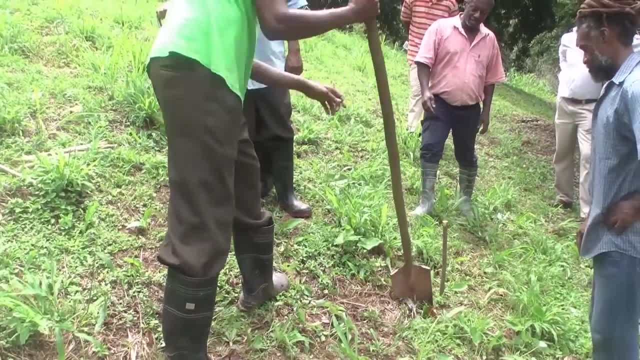 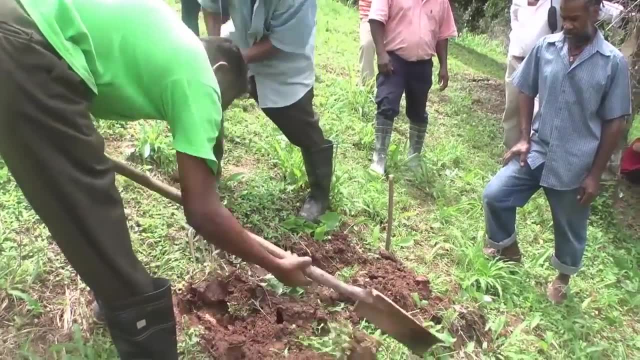 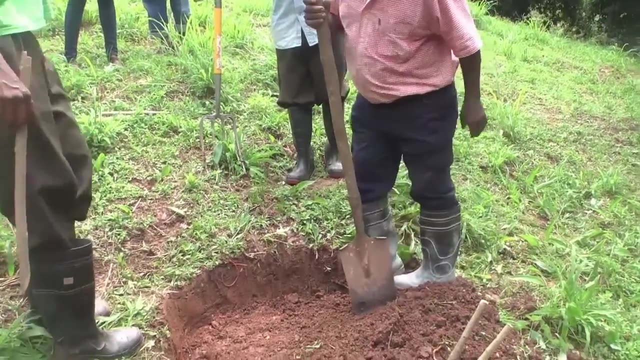 These are used for the purpose of planting long-term forest trees, fruit trees. You're trying to guess. You're trying to guess the best. You're trying to guess the best. The best area to plant the tree would not be at the edge of the loose soil. 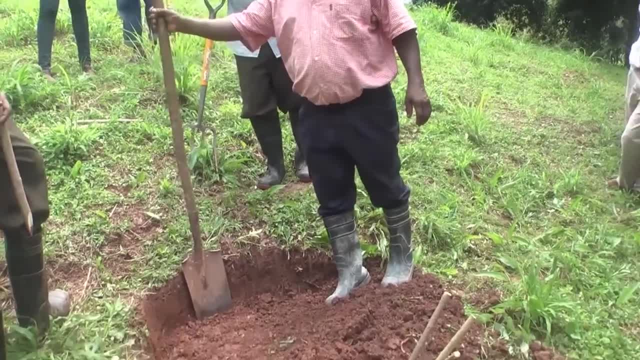 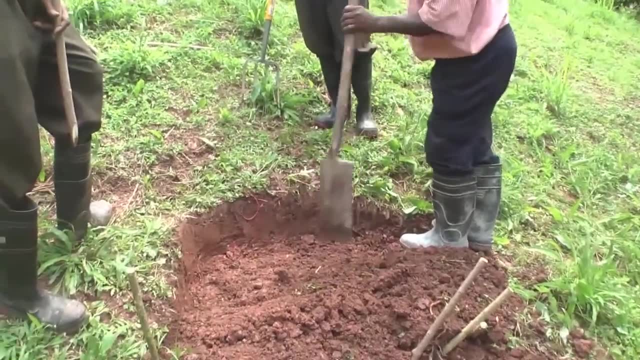 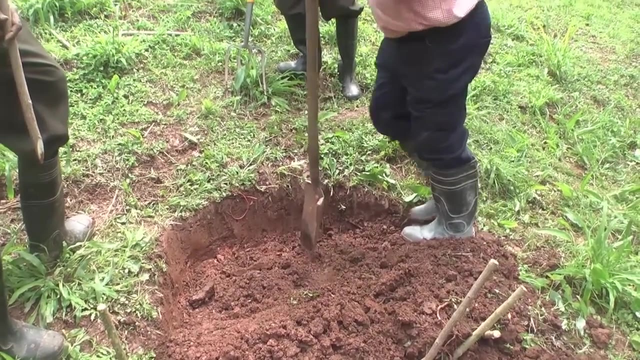 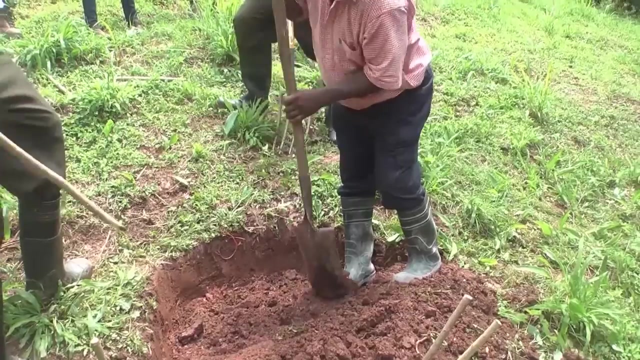 and would not be at the bank. here, where the soil is very thin, You'll plant it in the middle here, So we're going to dig a hole, Right. How many more? yeah, So you could take out three of the trees, right? 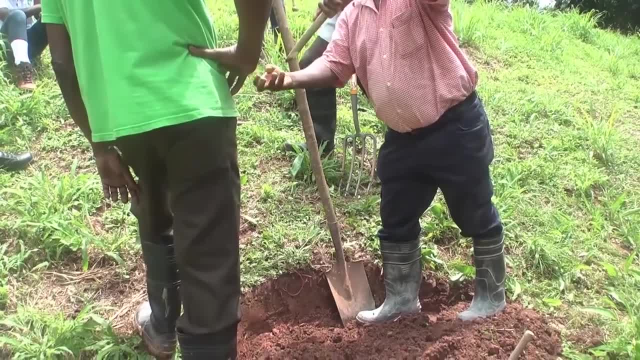 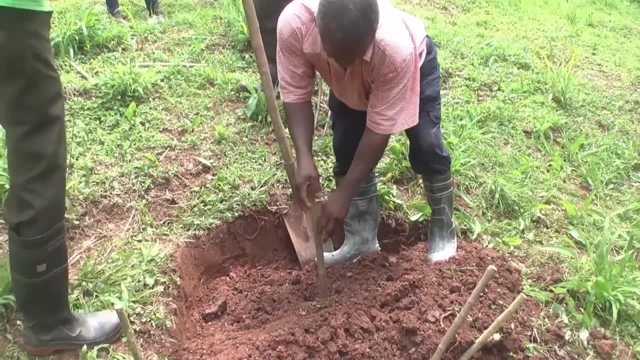 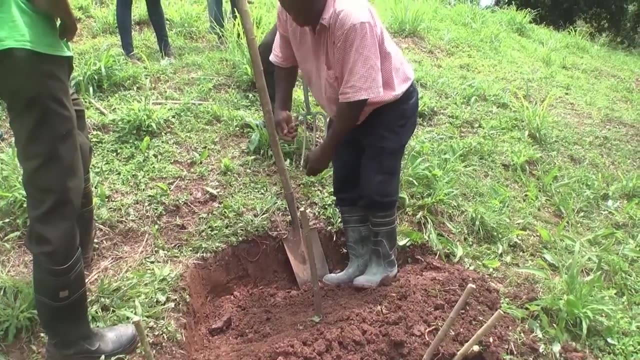 Take out the bag from this one. You've already got about three of them. You've already got about three of them. Put that tree there. Everything dries in- and help with that little water. Yeah, for some moisture. So when I go home I'll put some on the bed. 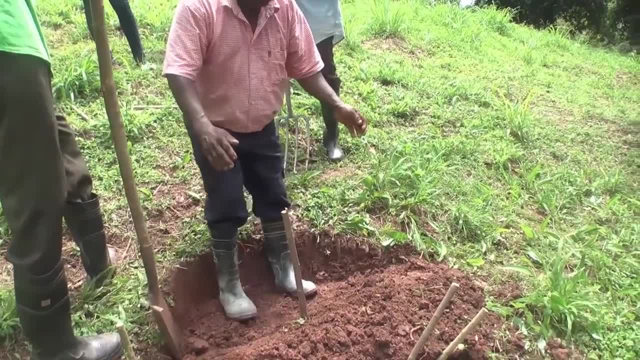 And the rest are gonna be getting dried out And the rest will be getting dried out. So I'll put some on And the rest will be getting dried out. You sprinkle it at the back here. The reason for this is to get your little manual and, wherever assistance with the fertilizer and what not. 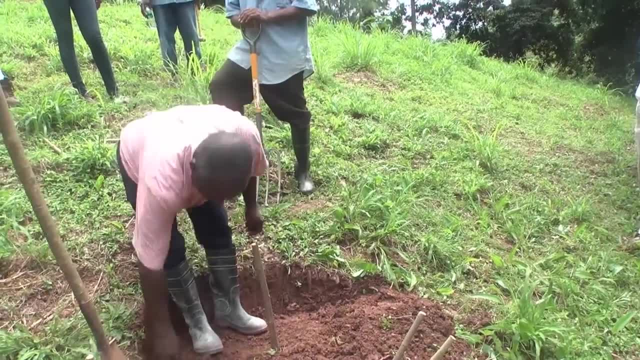 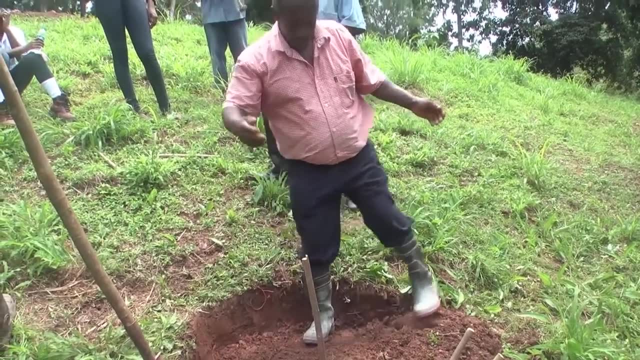 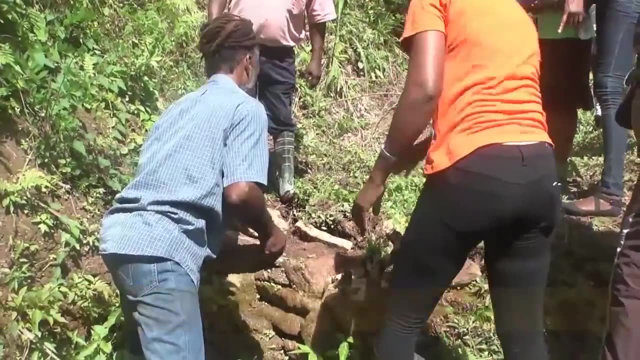 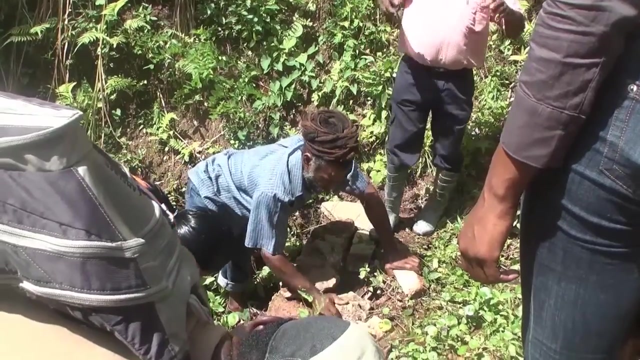 If you put the fertilizer here it will wash away. You sprinkle your fertilizer wherever your manual And you get your plant there. Start from the bottom there to come up behind that, there behind the grocery store. Yeah, right there, Get some of the heavier ones to the top. 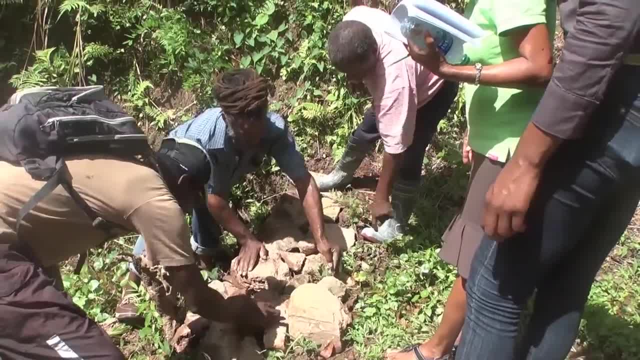 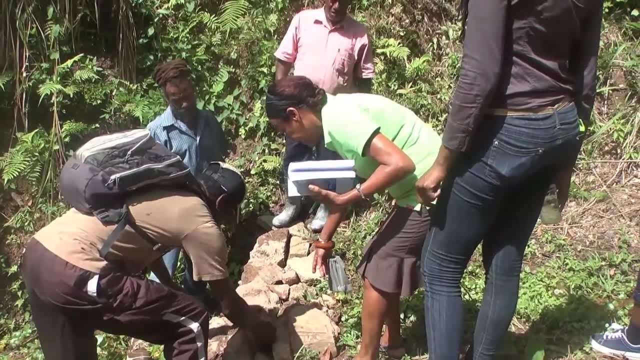 Get 15 of them And others in that little area. Lovely Right, And you have missed it. but where do you get your stones from? We get stones from around the area. In the event of no stones, you can use brick, concrete blocks. 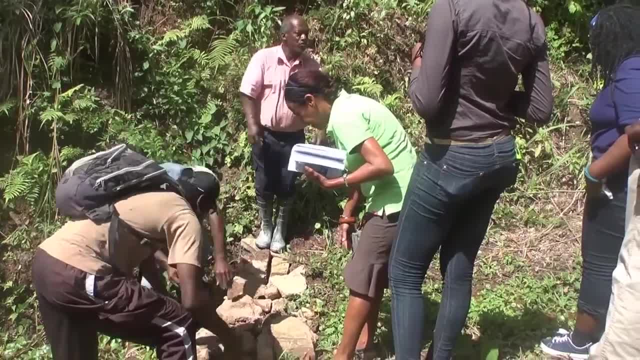 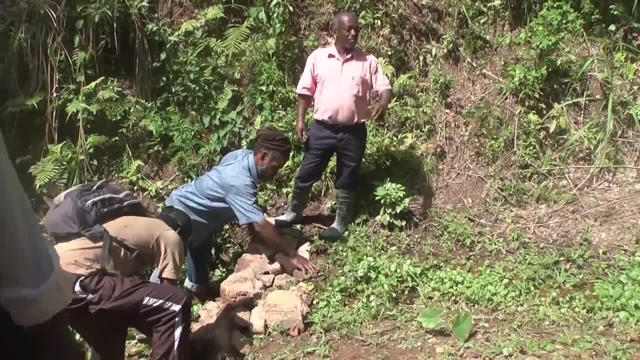 You get the concrete blocks. you get it cheap. You can use the same way, Right. so there you have it: The construction of a stone check dam by members of the group. This is how it is done: You start from the base. 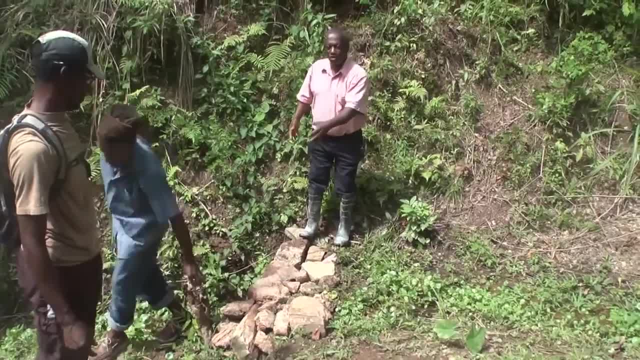 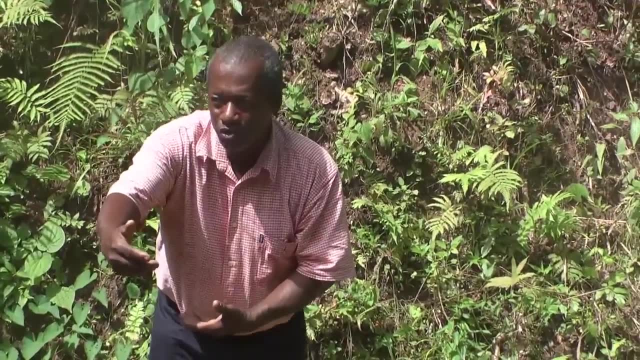 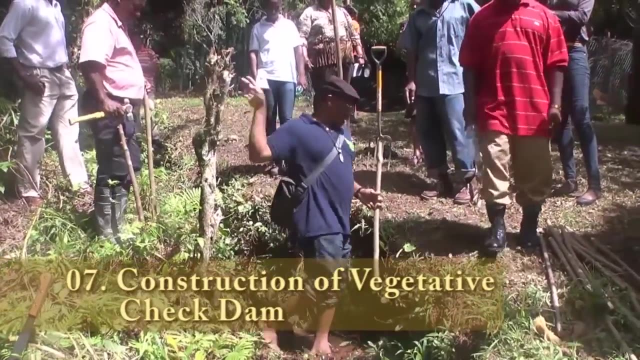 Some of the big stones from the base, the largest ones. Then you interlock some of the medium size and smaller ones coming up And you want a few large ones at the top To hold back the force of the water. The forestry will buy a shoe from me after. 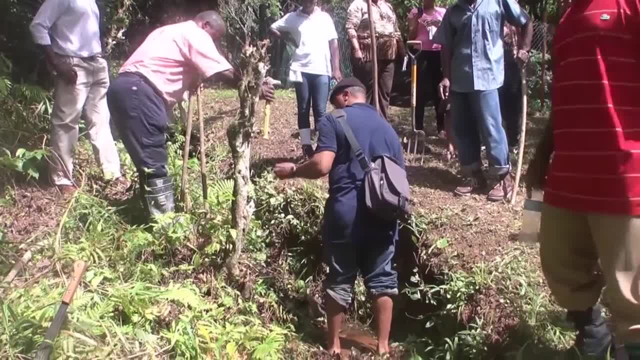 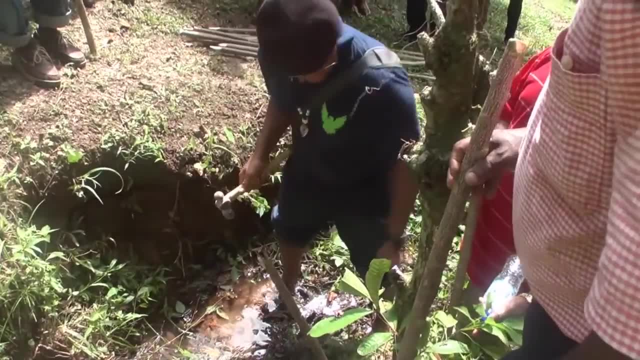 Oh man, I am thinking of my item size. Wait, wait, wait. Do you want from here? He said they're more than good. That's right. How about them all? You go in here. Let me put my hand in this. 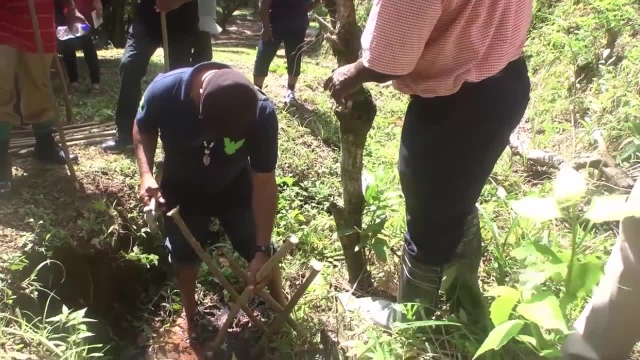 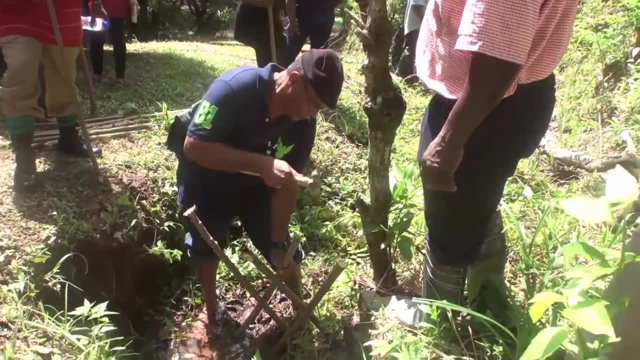 All right, that one here now. You can plant that one on the inside or on the outside, Children, it doesn't matter. That might be better, Right, So you can take an X boat with you Here. My question is: